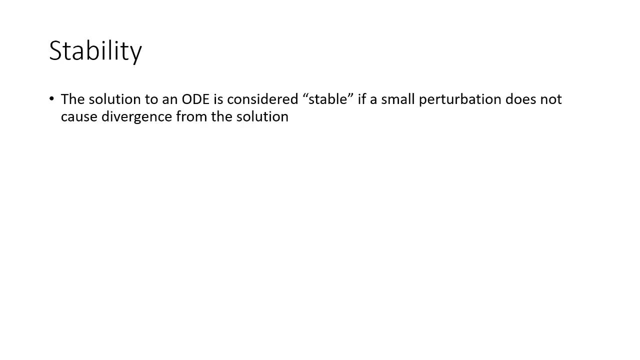 So first we need to define stability For the case of an exact solution to an ordinary differential equation, that exact solution is considered stable if a small perturbation does not cause a large divergence from the exact solution. Now for a numerical method. the method itself is considered stable if a small perturbation does not cause the numerical solution to diverge without bound. 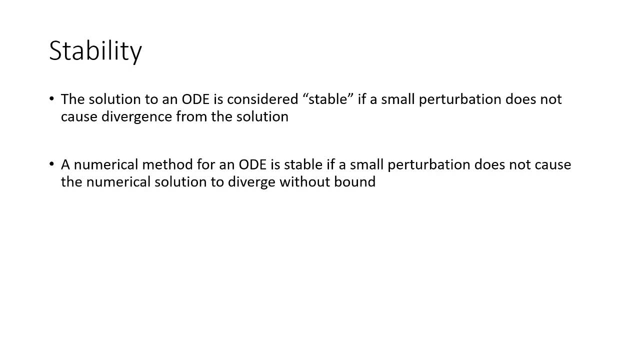 So think about this: If the numerical method solution is going to go to infinity, that's an unstable solution. In order to discuss this, we're going to consider the following first-order ODE with an initial condition of y-not. It's going to be: y' equals lambda y, where that lambda can be any real or imaginary value. 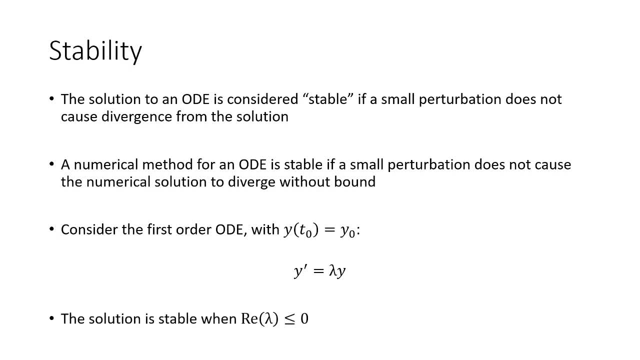 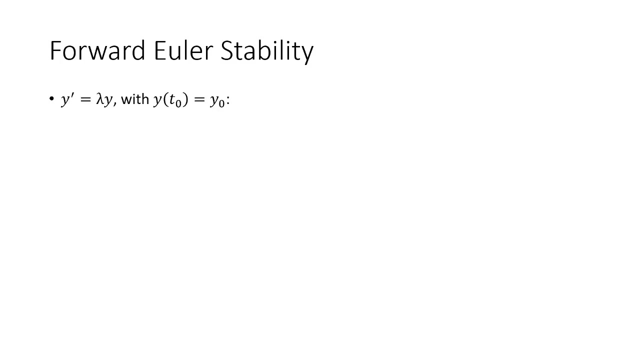 Now the exact solution to this ODE is stable when the real value of lambda is less than or equal to 0. So if lambda is positive, your solution is going to go to infinity right. So then, the exact solution is unstable. Now let's talk about the stability conditions for the forward Euler method for this ODE. 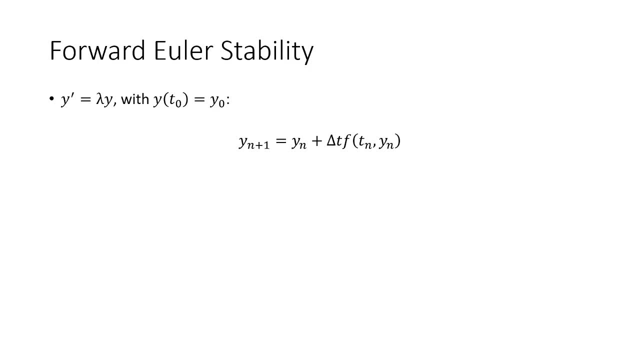 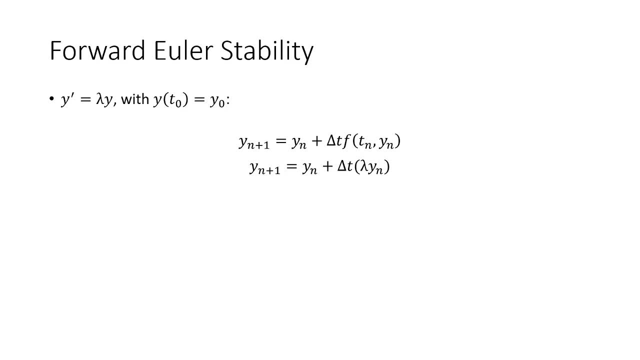 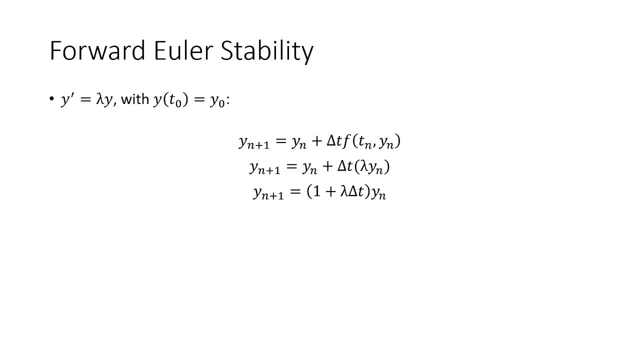 of y sub n. So this is our general explicit solution here. Now let's consider the case where n equals zero. So if n equals 0, y of 1 equals 1 plus lambda delta t times y0.. Now if we're trying to solve for y of 1, it would be like this: 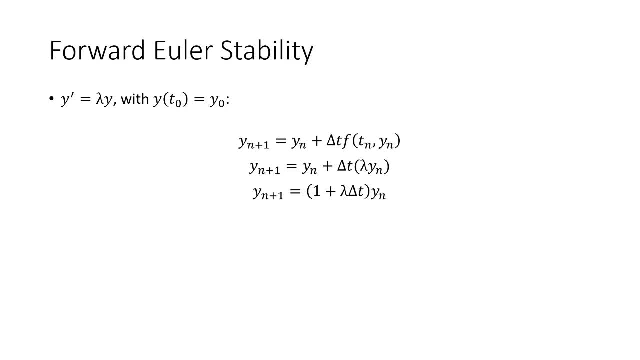 Now if we're trying to solve for 1, it would be like this: y2 is going to be equal to y1 times 1 plus lambda delta t. So you can see the pattern here. For each additional step in our solution, we multiply the previous step by another 1 plus lambda delta t. 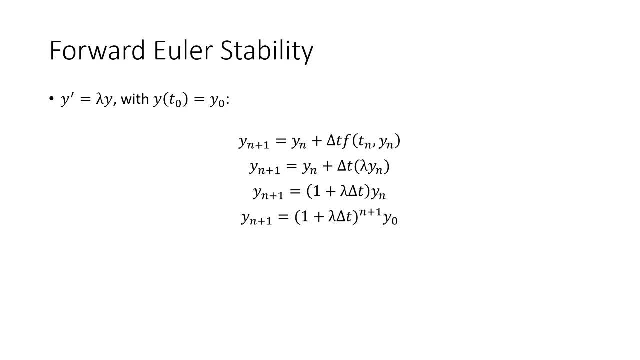 So the solution at any time step based solely on lambda delta t, n and y naught, looks like this: y sub n plus 1 equals 1 plus lambda delta t to the n plus 1 times y naught. So this solution is going to be stable when 1 plus lambda delta t is less than or equal to 1.. Because if that product 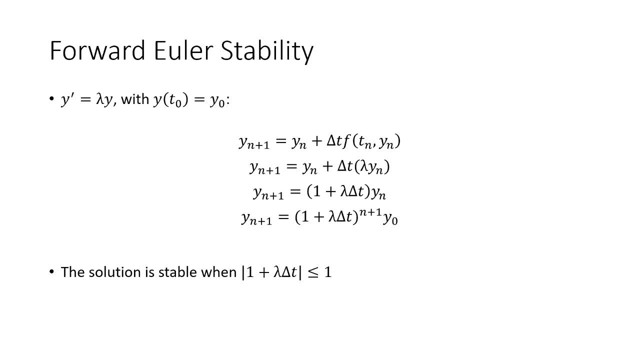 or if that quantity is greater than 1, then our solution is going to infinity. y sub n plus 1 is going to just keep getting bigger and bigger and bigger. So before we go ahead, this is important because lambda is going to be given to us for a given- 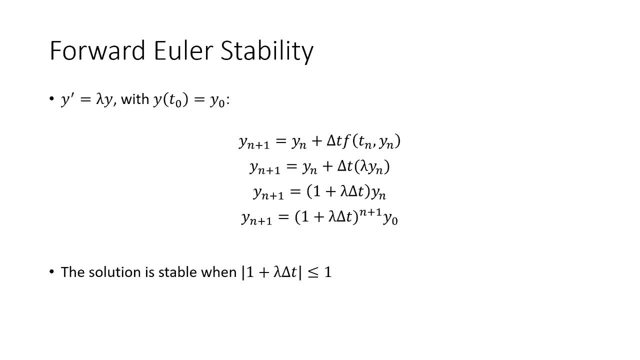 problem. But we get to choose our delta t. So if we know this stability condition, it helps us select a proper delta t for a stable numerical solution. So we're going to do a similar thing for the backward Euler method. Here's our backward Euler equation. We're going to plug in our function, It's going to be lambda of 1.. So we're going to do a similar thing for the backward Euler equation. We're going to plug in our function. It's going to be lambda of 1. So we're going to do a. 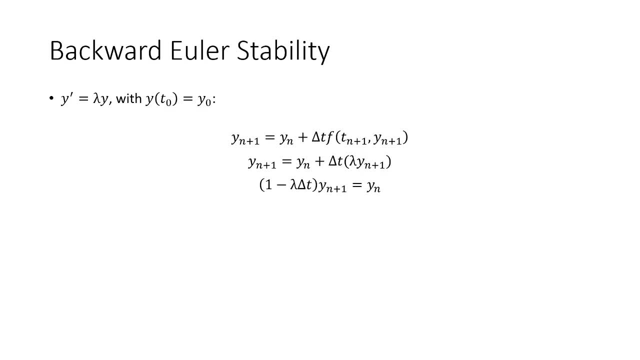 same method again, but with a little effect. Now I'm going to go out and we're going to make our backsuit circle, So we're going to make the back shape circle. If it'sbulaT that's going to do the same thing, We're going to divide that by 1 minus lambda delta. 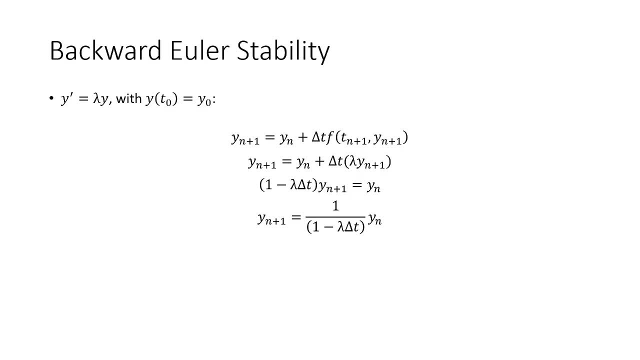 t, And then we're going to make that substitution of y naught into our final answer, so that we have an equation for y sub n plus 1 at any time step. So now you're going to see that it is this quantity here that has to be less than or. 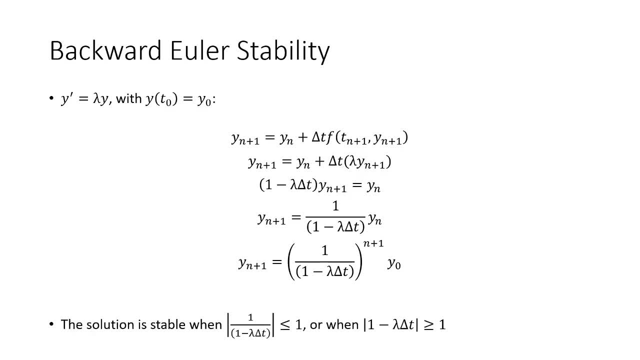 equal to 1.. 1, this 1 over 1 minus lambda delta t. So that's our stability condition for the backward Euler method. It's stable when the absolute value of 1 over 1 minus lambda delta t is less than or equal to 1.. We rearrange that It's stable when the absolute value of 1 minus. 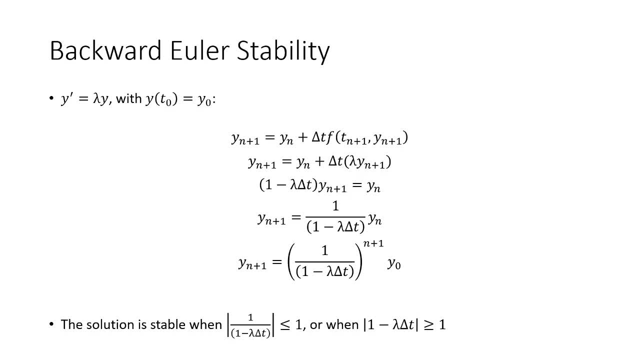 lambda delta t is greater than or equal to 1.. So an interesting and different stability condition from the forward Euler method, But again it gives us insight into a proper delta t. So finally, the trapezoidal method. stability is slightly more complex, since we're going